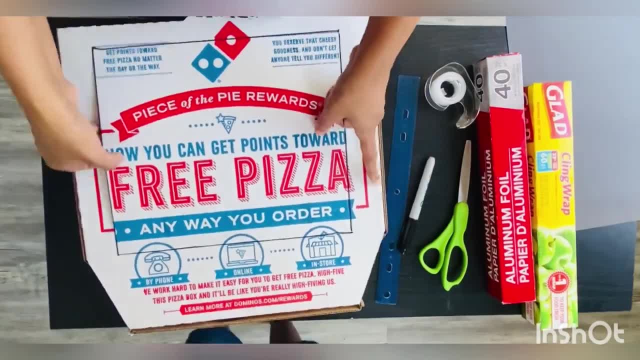 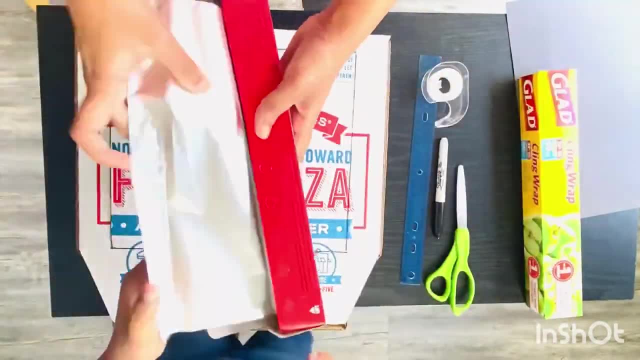 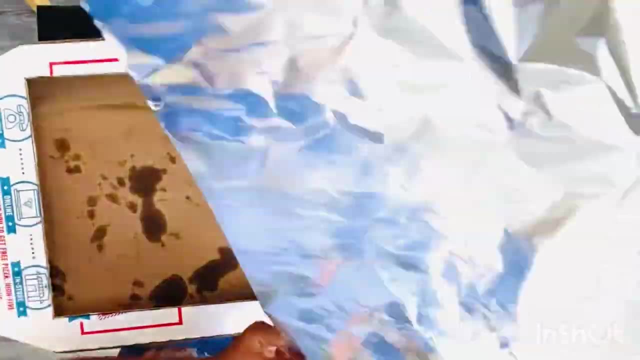 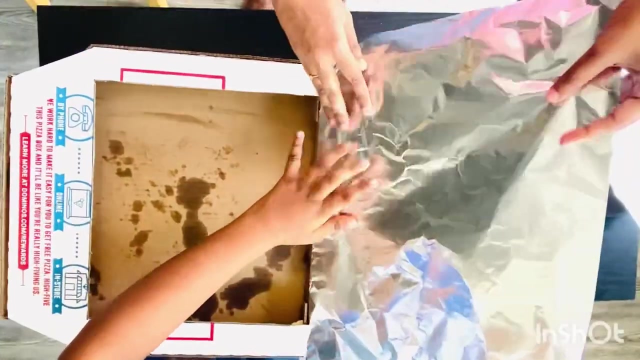 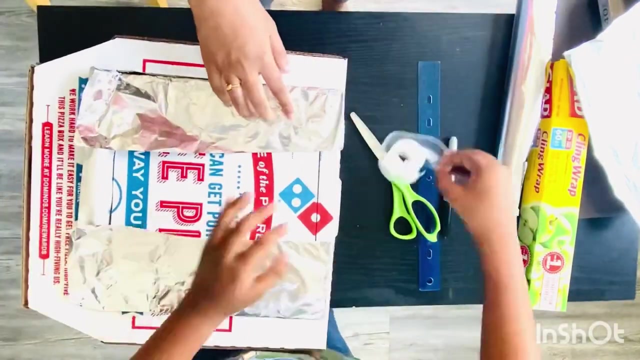 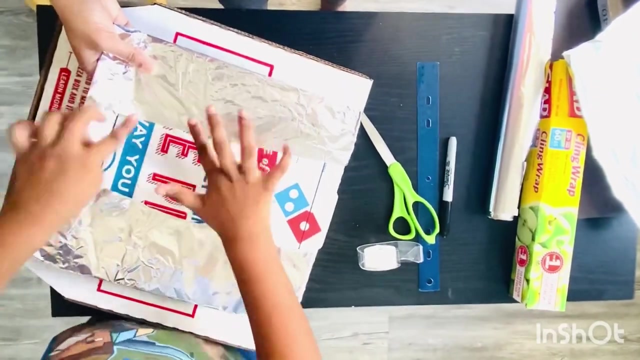 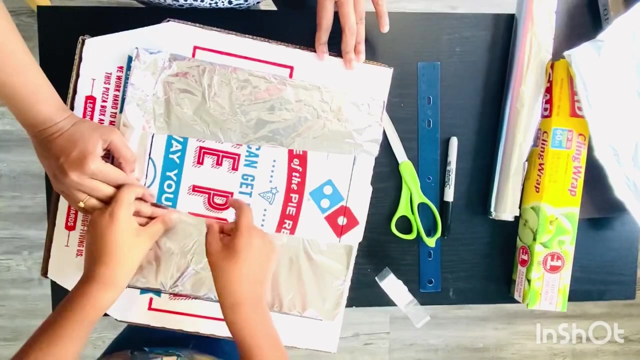 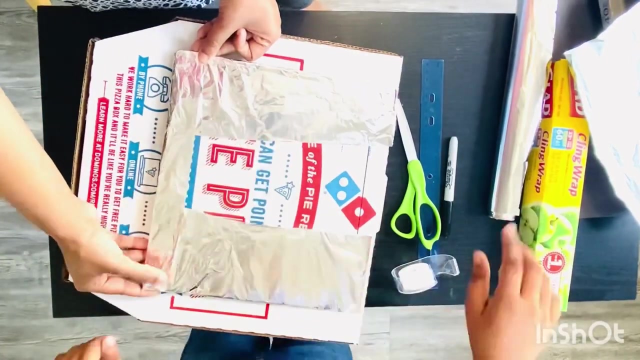 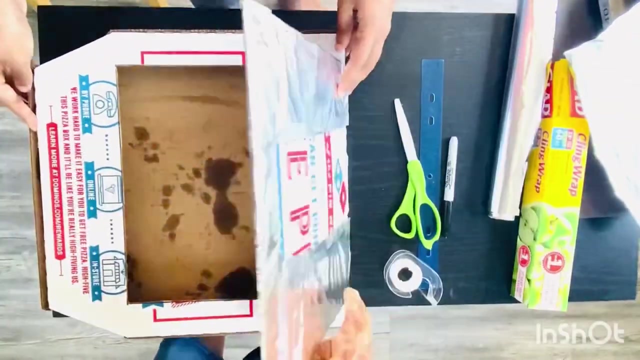 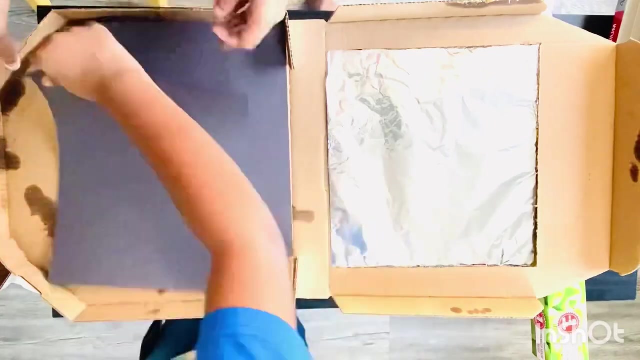 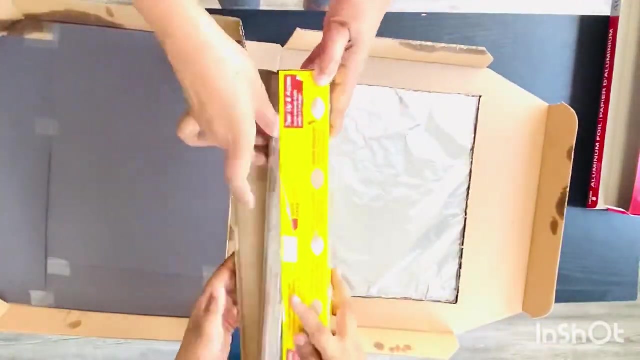 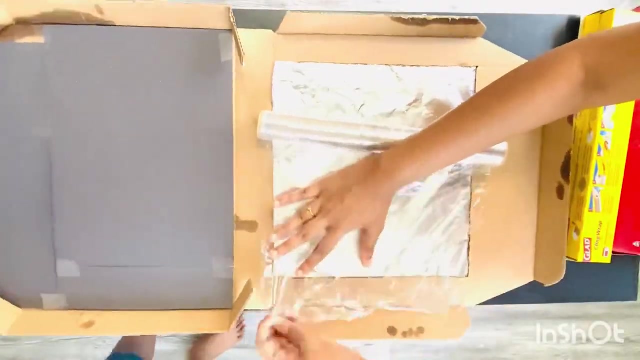 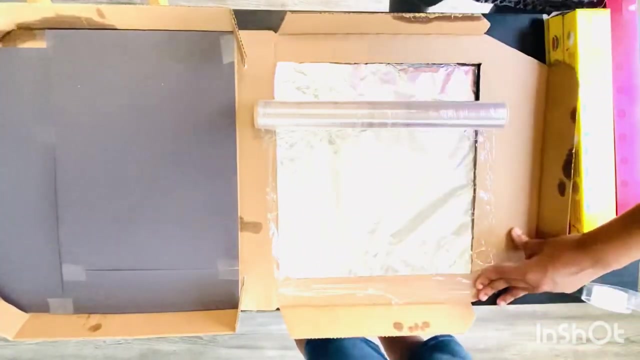 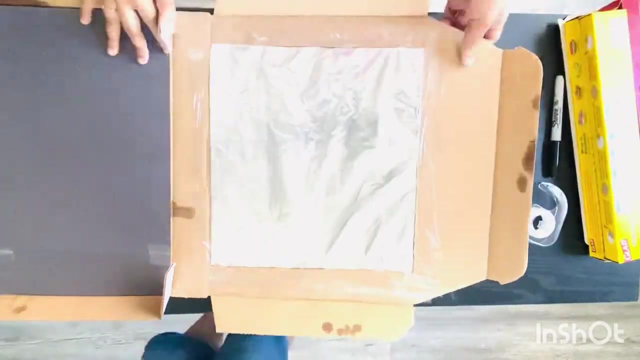 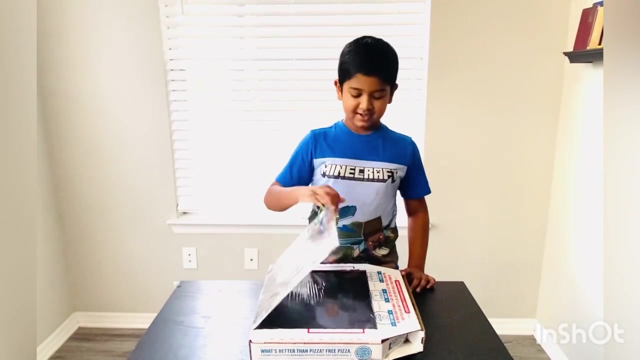 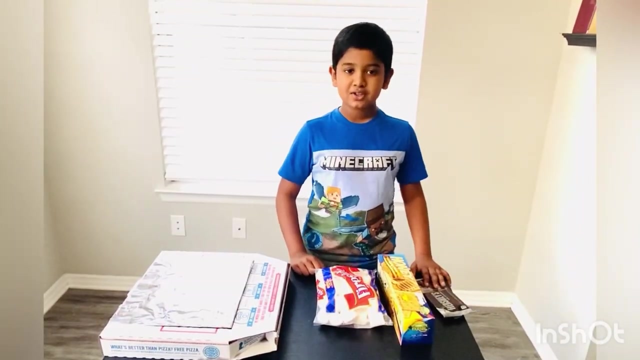 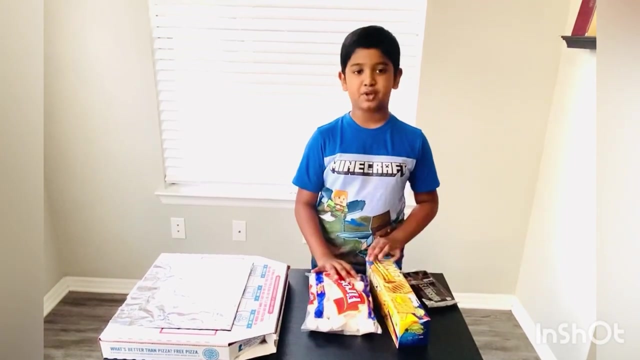 Let's get started. Let's get started. Let's get started Now. our solar oven is ready. Now let's make a s'more. To make a s'more, we will need Hershey's chocolates, graham crackers and jumbo size marshmallows. Let's make a s'more. 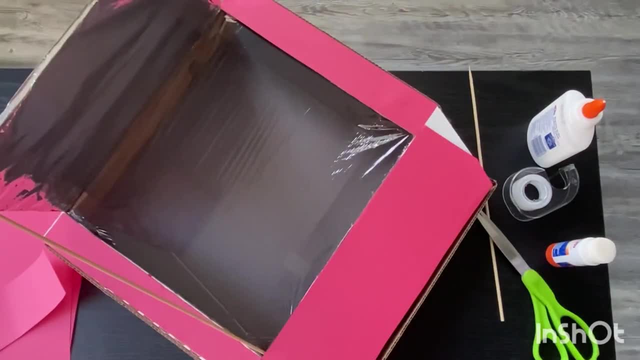 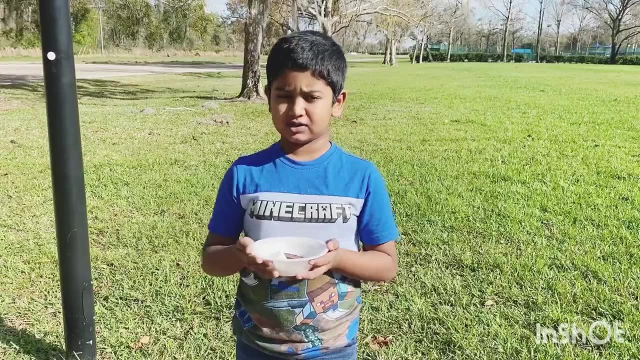 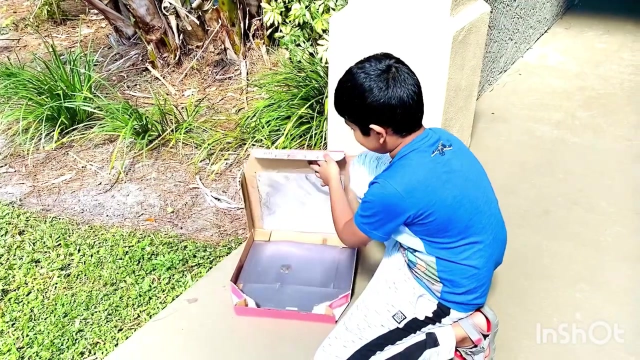 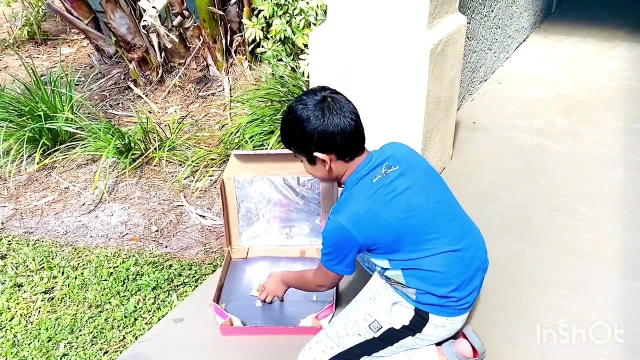 So now we will come out to make our s'more, So let's go and keep our s'more inside our solar oven. So first, if you should keep the s'more inside the fridge And put it in the fridge, 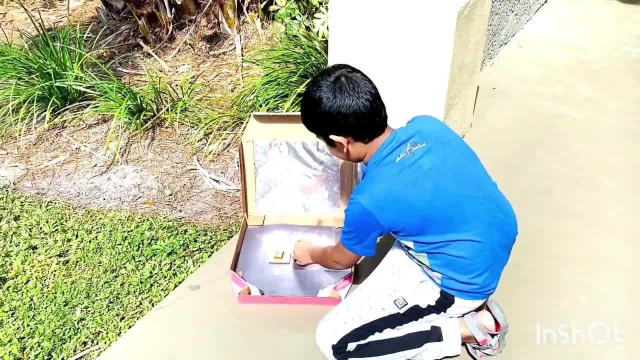 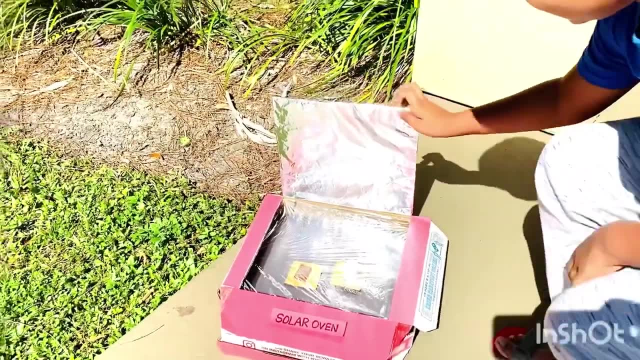 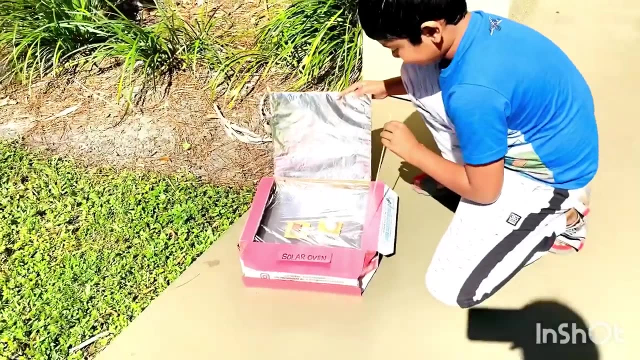 Okay, Okay, Okay, Okay Okay. All right, This is all set out. Beats this here. Now we're going to wait for our chocolate and marshmallows to melt. Let's keep this as a stand for our solar oven.